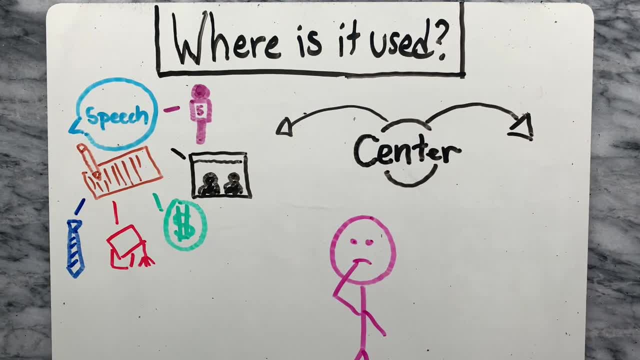 In political talk, you'll often hear people use the political spectrum to signify a person or policy while trying to find common ground. For example, a politician might be accused of being too left-wing, or a media outlet might be known as right-wing media. 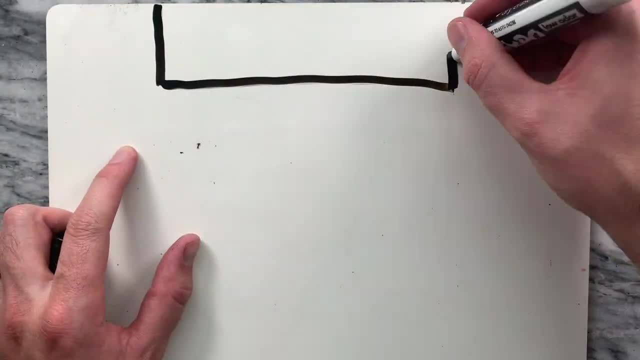 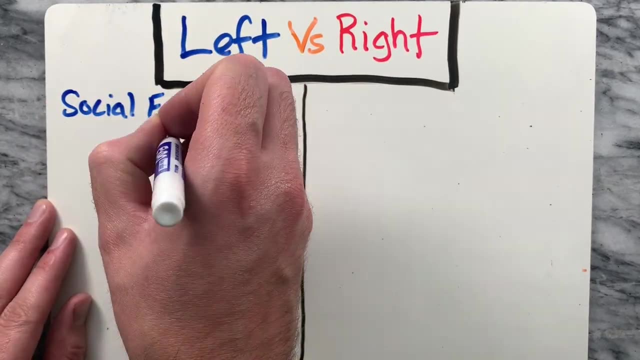 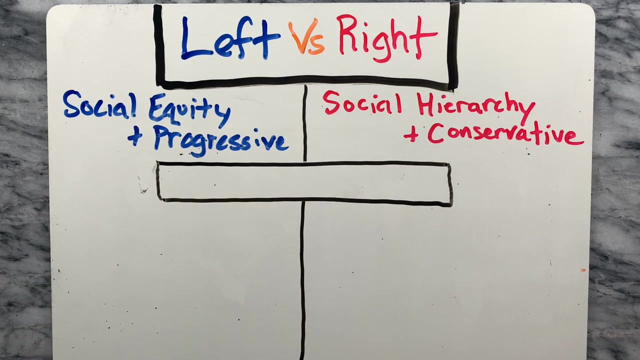 So what exactly does left and right mean? Let's take a look at that next. The left-right political spectrum is used to describe political positions, ideologies and parties, from social equality and progressive ideologies on the left to social hierarchy and conservative ideologies on the right. 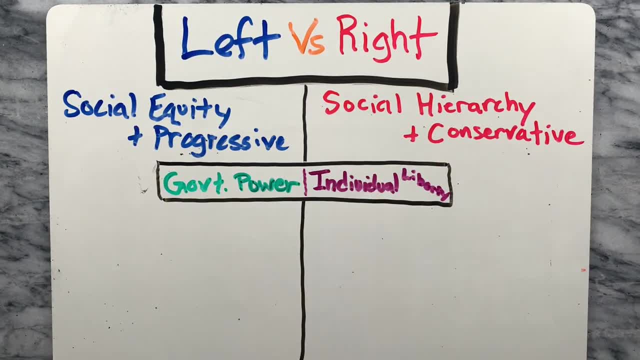 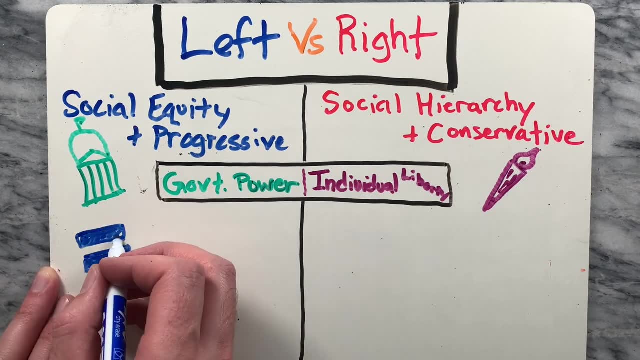 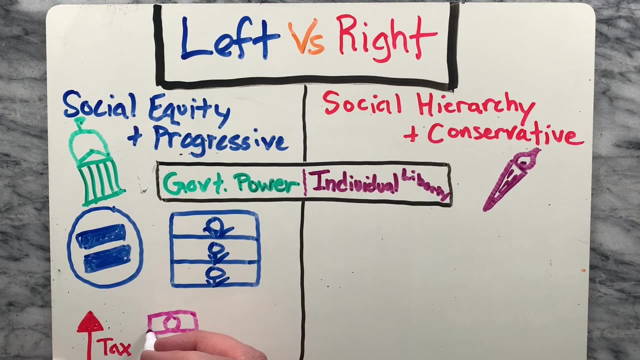 For example, if we look at the balance between government power and individual liberty. the left would strive for an equal society and support the government playing a large part in people's lives. in order to achieve this, They tend to support higher taxes on the rich, welfare for the poor and government regulation. 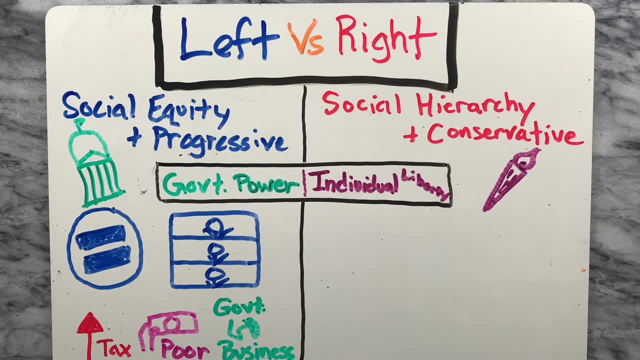 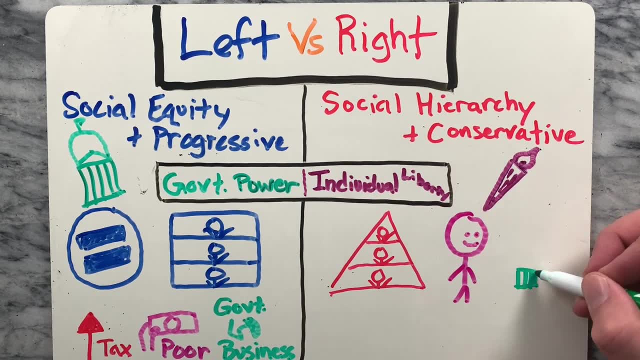 of business and the economy. If we take a look at the right-right political spectrum, we'll see that the left-right political spectrum is the right. The right would say that a certain level of social inequality is unavoidable and that the government should play a limited role in people's lives. 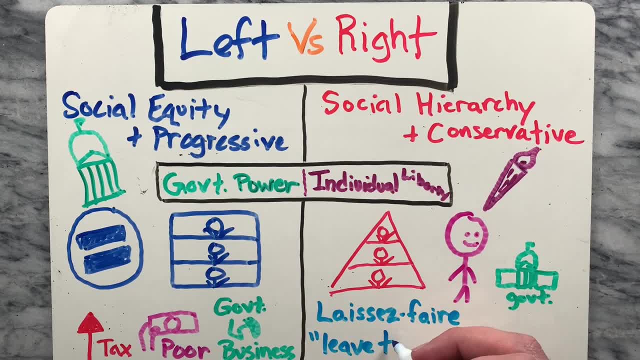 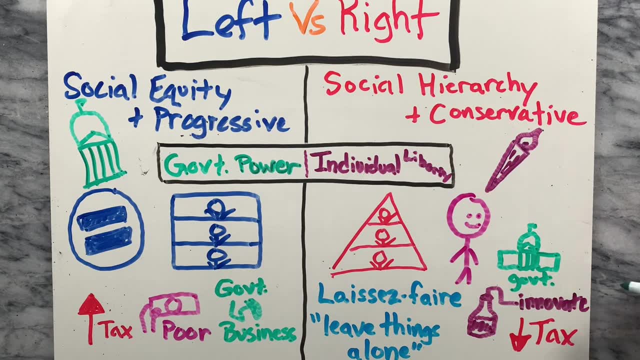 They strive to support a laissez-faire approach to the economy. Laissez-faire is a French term which roughly translates as leave things alone. Those on the right believe that less business regulation will help innovation and lowering taxes on businesses will help them grow. 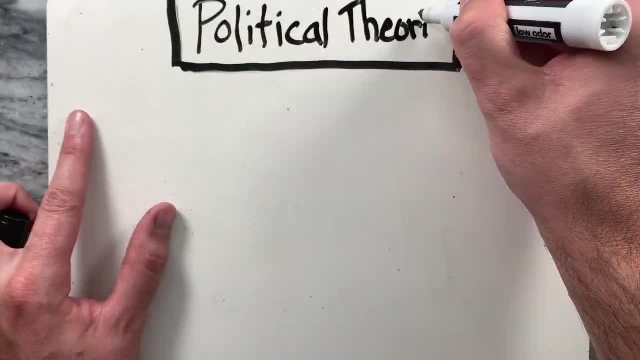 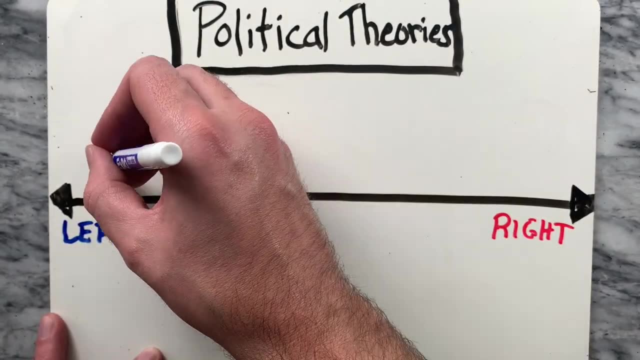 Now let's look at some political theories and where they sit on the left-right spectrum. When looking at political theories like communism and socialism, the left-right political spectrum would be placed in differing degrees, because they support social organization that is owned or regulated by the community or government. 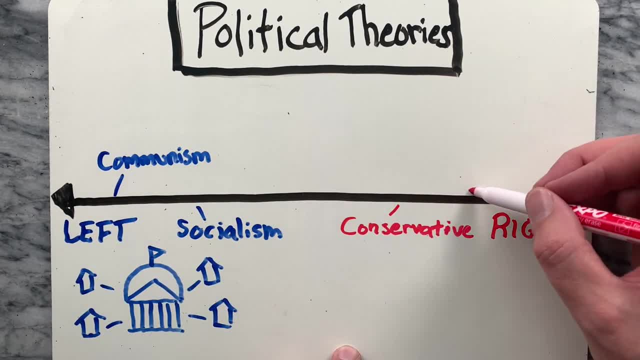 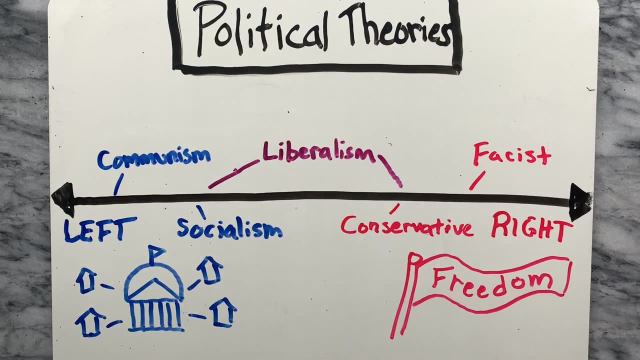 Conservative and fascist theories are typically regarded as being on the right because they support varying degrees of nationalism and independence, Then liberalism can mean different things in different contexts, with social liberalism on the left and conservative liberalism on the right, and those in the middle are classified. 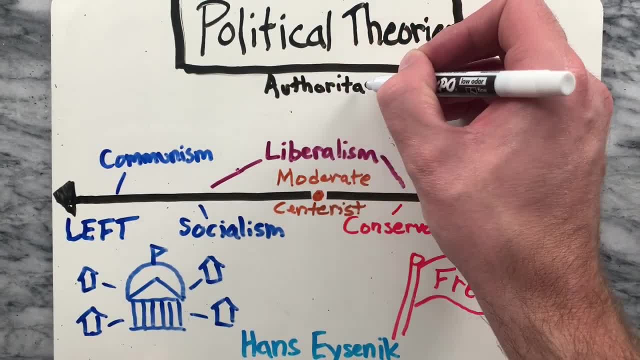 as centrists or moderates. Many argue that a one-dimensional spectrum is too simplistic. They use the term social liberalism as a metaphor. considering the patriarchy that educates the, Hans Eysenck, a German-born British psychiatrist, made a model that added a second axis to the. 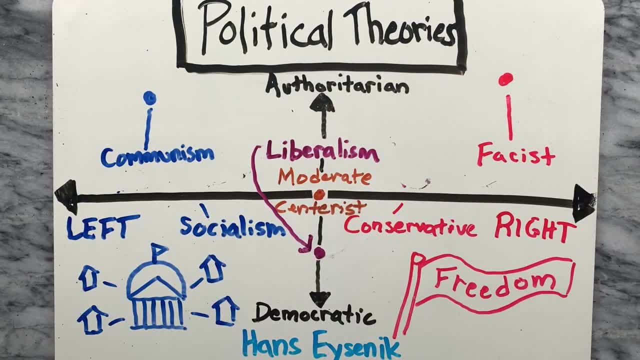 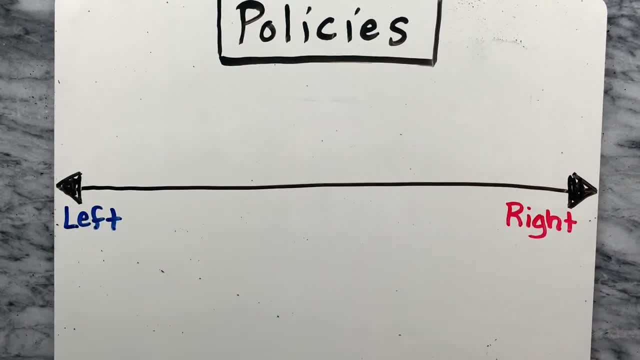 political spectrum with authoritarian and democratic dimensions to better place political theories. Next let's look at a couple examples of policies and where they are positioned on the spectrum. An example of a policy on the left would be Sweden's Parental Leave Act in 1974.. 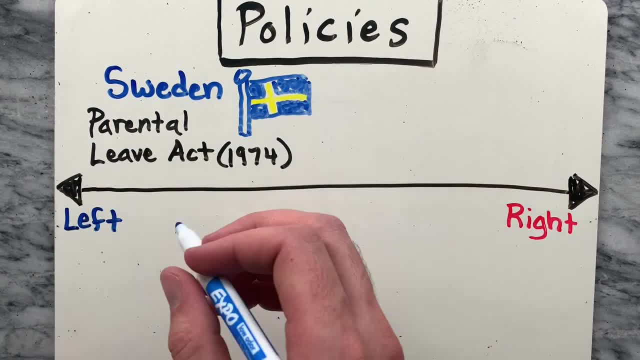 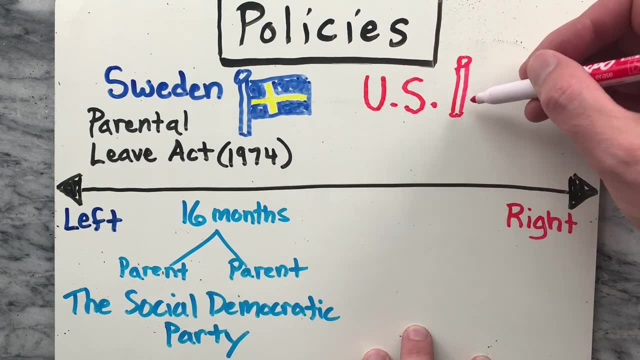 Sweden became the first country in the world to introduce parental leave that could be split between two parents of a child. It was pushed forward by the Social Democratic Party, which is known to pass progressive policies on social change. An example of a policy on the right would be the United States Tax Cuts and Jobs Act. 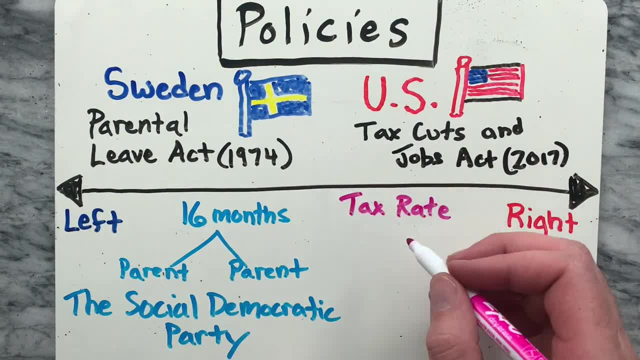 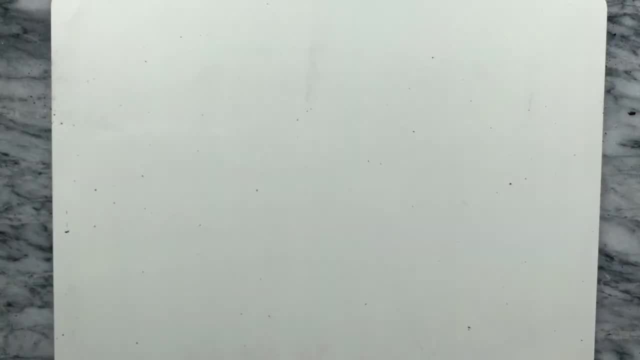 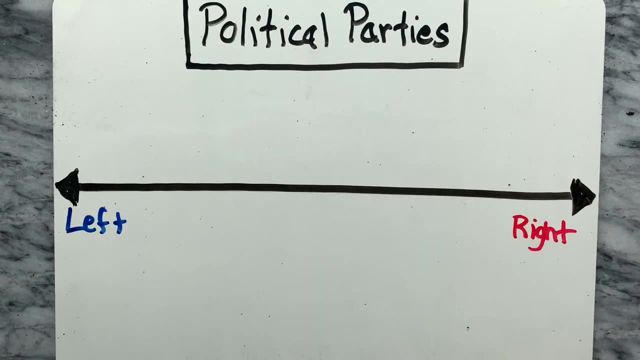 in 2017, which reduced tax rates for businesses from 35% to 21%. It was implemented by the Republican Party, which generally supports laissez-faire economics. What about political parties? On the left wing, you'll find parties like the Democrat Party from the United States. 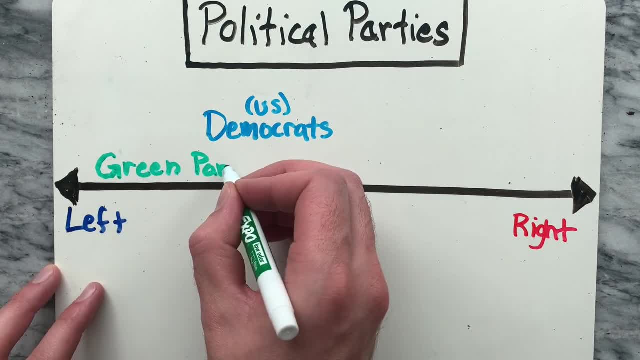 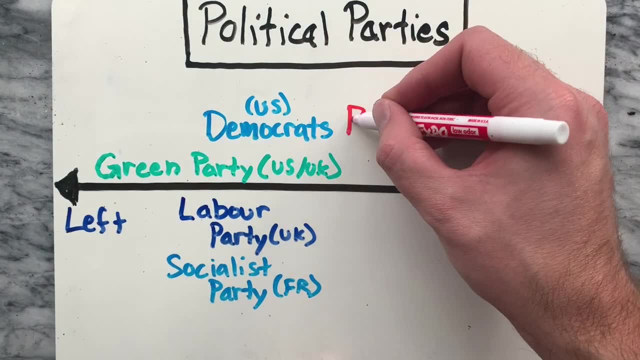 the Green Party from the United States and the Democratic Party from the United States, The Democratic Party from the United Kingdom and the United States, the Labor Party from the United Kingdom and the Socialist Party from France. Right wing parties include the Republican Party from the United States. the Constitution. 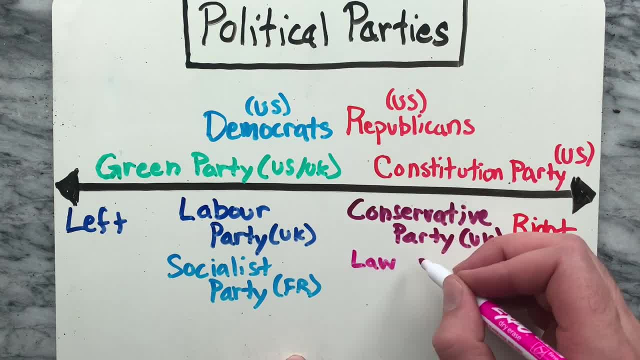 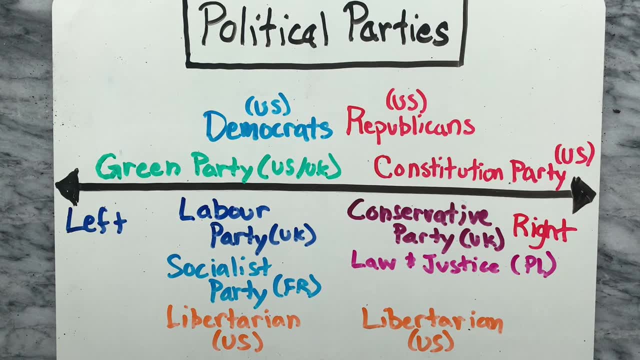 Party from the United States, the Conservative Party from the United Kingdom and the Law and Justice Party from Poland, and, lastly, the Libertarian Party can be placed on the left or the right, depending on the topic. It's important to remember that it's not all black and white. 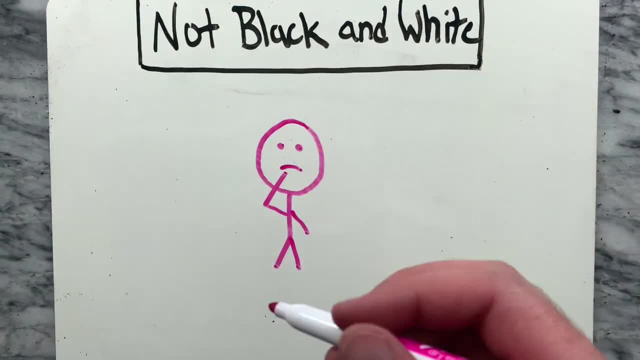 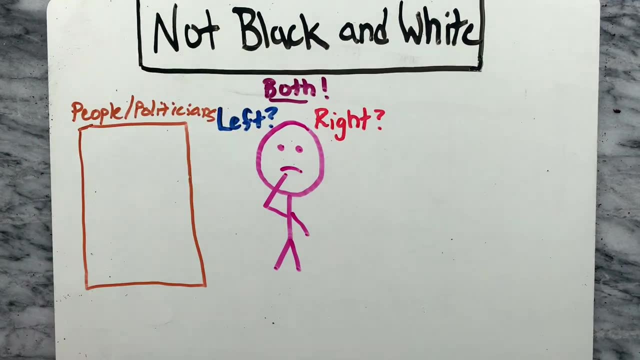 It's not all printed, It's all different. Many principles, laws, political parties or politicians can be neatly classified as left or right wing, as most will include elements of both. Likewise, politicians even those who describe themselves as being left wing or right wing. 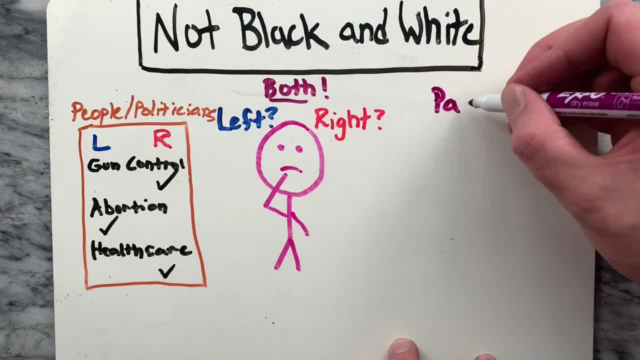 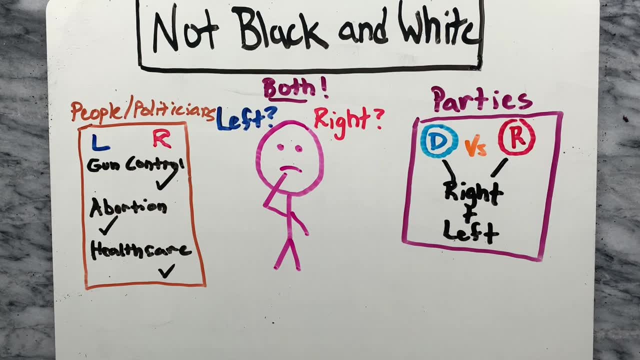 will often support one or two principles from the other side of the spectrum. For example, many policies for both the Democrat and Republican Party could be considered right or left wing. Likewise, a political party might become more left or right wing depending on its leader. 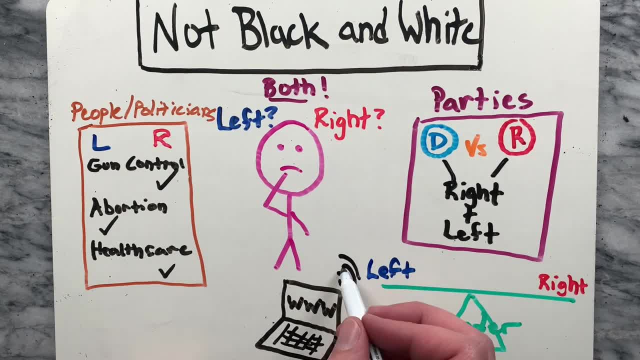 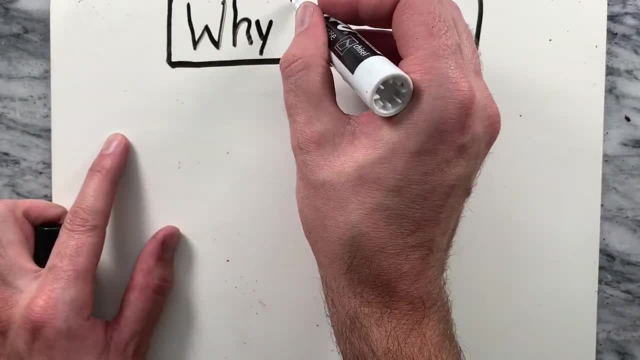 at the time. It's not always specific. Whether you like it or not, you're in the right or left wing field party's actual platform. before making up your mind on who to vote for Now, you might be wondering: why does any of this matter? It's useful to have an